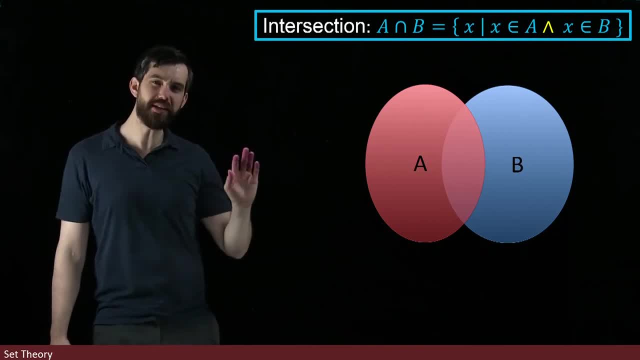 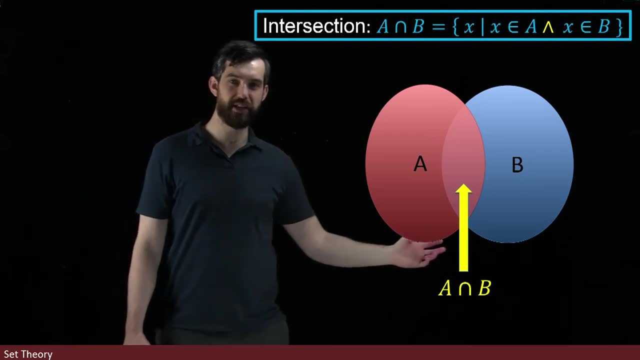 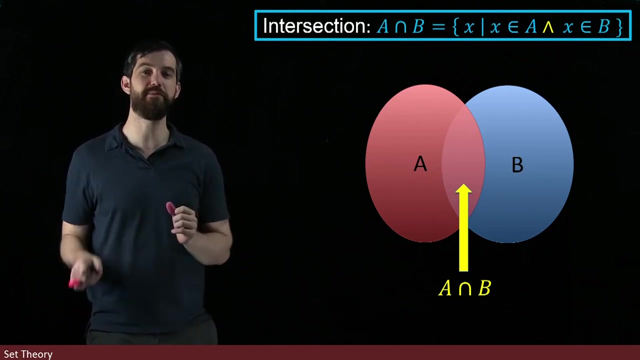 overlapping. so there's something interesting: If I want to say that X is in both A and B, then the intersections, that that bit in the middle here, this, this portion is sort of overlapping the, the shaded region in the middle where they are both in the A and the B. that's the idea. 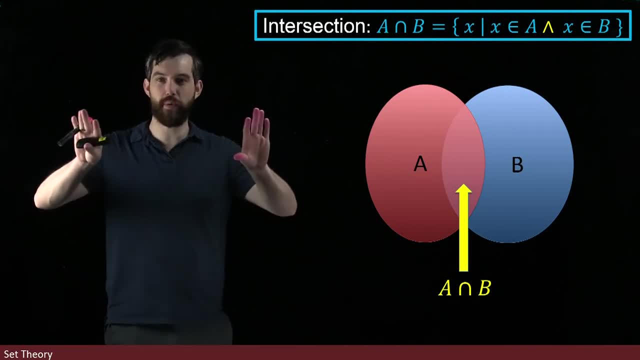 of the intersection. If the A and the B, by the way, were completely separate, there wasn't any overlaps and the intersection would be the empty set, because there's no element that's going to be in both of them. So let's see an example of this Again. I'm 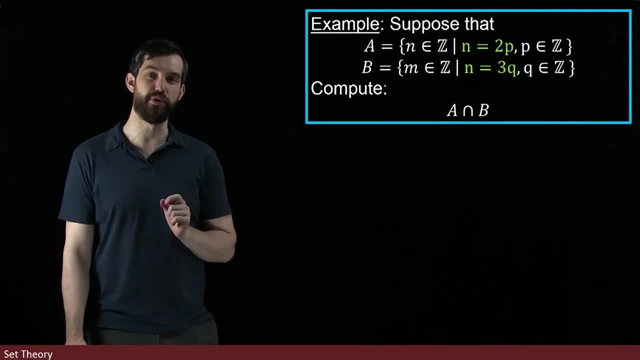 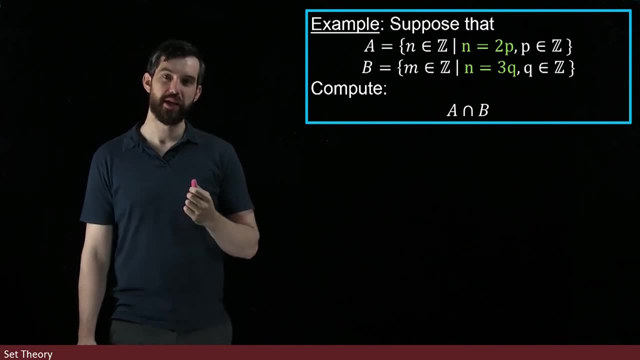 going to have an A and a B. Notice I've changed the A and the B on you again. The A is going to be N equal to 2p, so this is going to be all of the even integers. The B, however, is equal to N equal to 3q, and this is going to represent the. 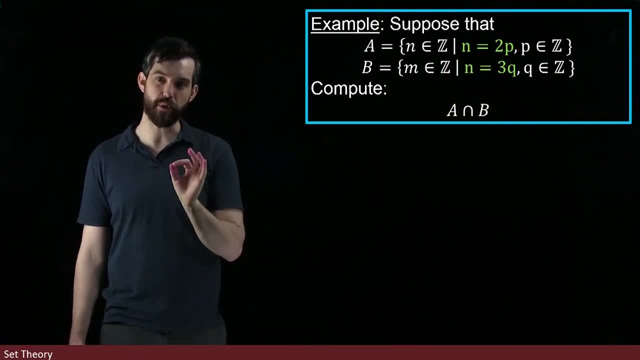 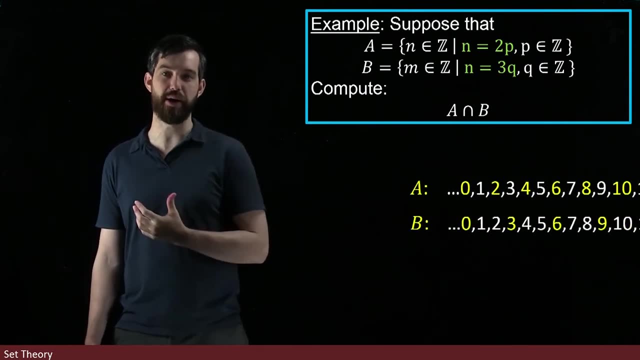 all multiples of q. So then, if I want to write it down, I can do the same trick, where I'm going to highlight the integers that are relevant. here, I'm going to highlight, in the case of A, all of the even integers 0,, 2,, 4, and so on. 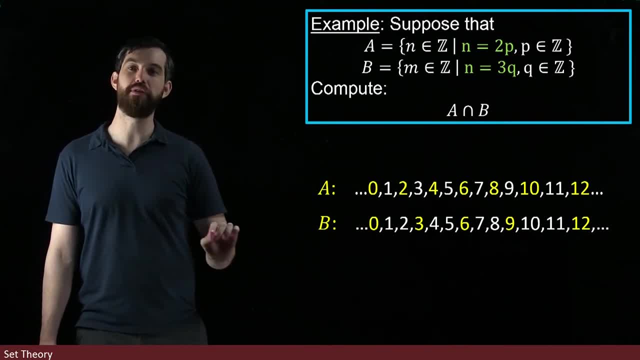 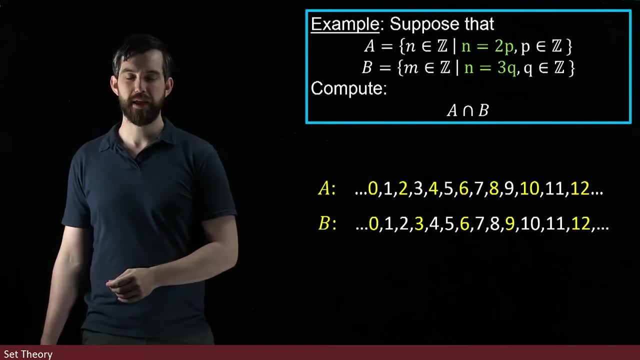 And, in the case of B, I've highlighted in yellow all of the multiples of 3.. 0,, 3,, 6,, 9,, 12 and so on. So, then, the intersection are the things that are in both the A and. 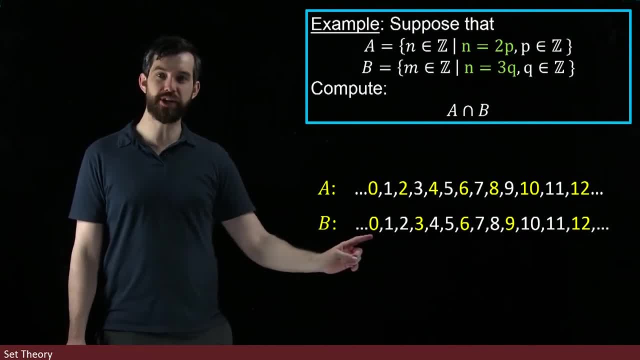 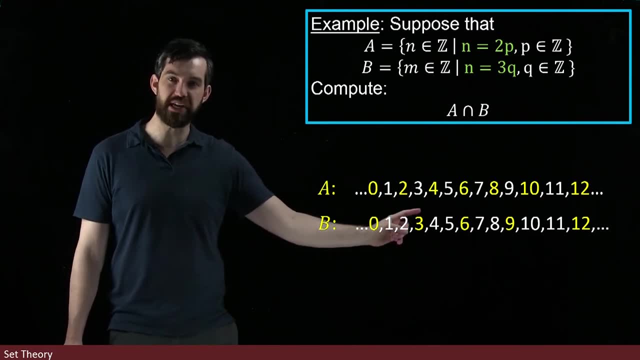 the B, So let's think about how that works. Okay, the 0 is in both of them, so that should count. The highlighted 2 here is only in A, The highlighted 3 here is only in B, The highlighted 4 here is only in A, But then the 6 is highlighted. 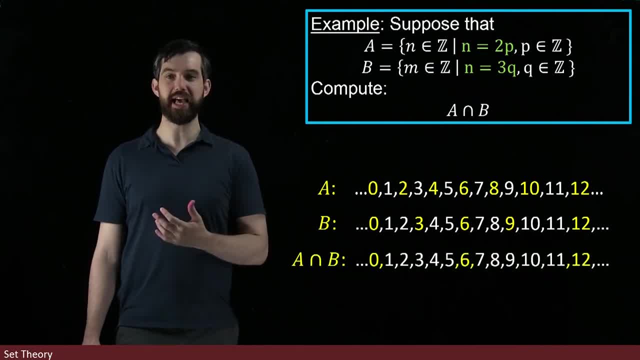 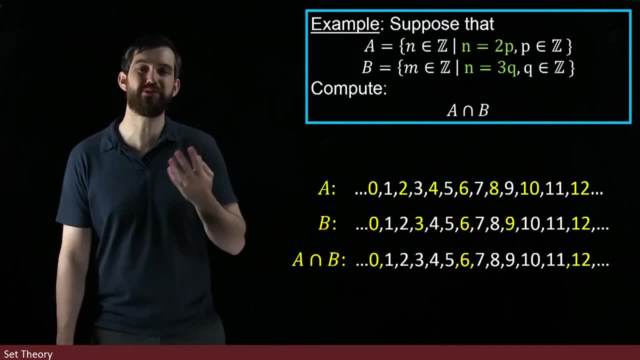 on both of them. So this looks like the multiples of 6, and indeed that's what A intersect B is going to be. It's going to be the 0, the 6,, the 12,, all of the multiples of 6.. That's what it means to be both a multiple of 2 and a. 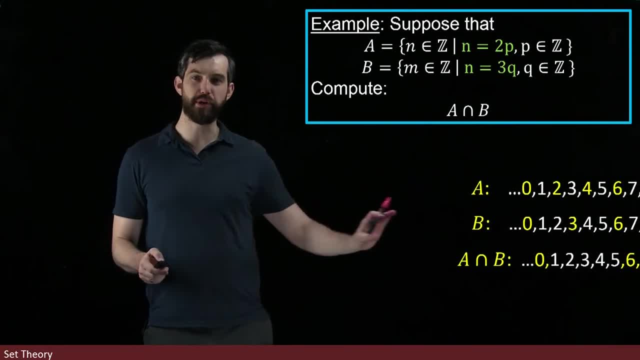 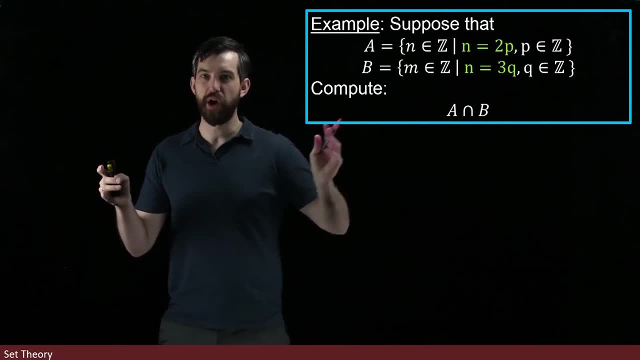 multiple of 3.. So now, if we're going to formally prove this, then I'm going to do the same trick as before. I'm claiming that this is going to equal all the multiples of 6.. So I'm claiming an equality. So that means that I want to. 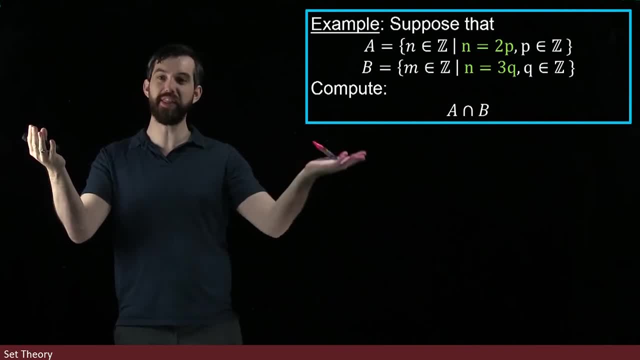 show. if I've got something in the one, it's in the other, and if I've got something in the other, it's in the one. I want to be able to show both directions. So the proof that I'm going to do is going to have biconditionals- logical. 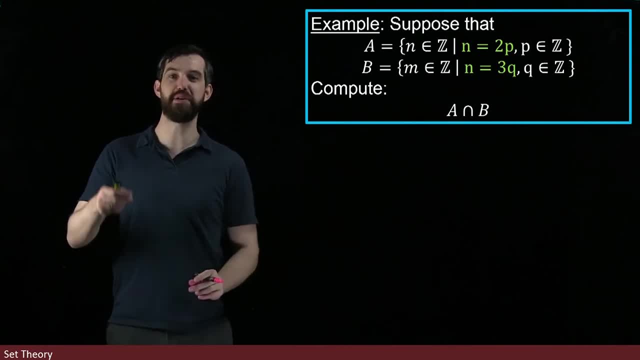 implications that work both ways, that every single step That tells me if I start in the intersection I'm in the multiples of 6, and if I'm in the multiples of 6 I'm going to end up in intersection. So let's start in the intersection, just doesn't really matter. we got to start somewhere. 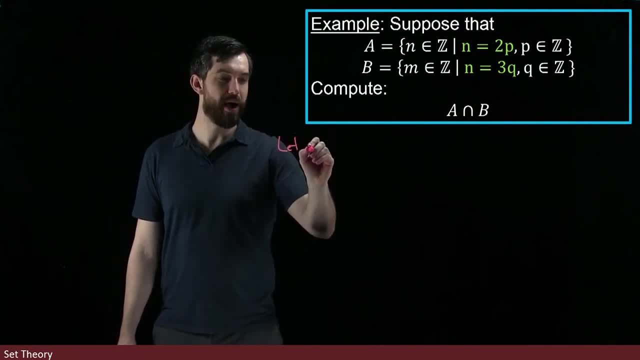 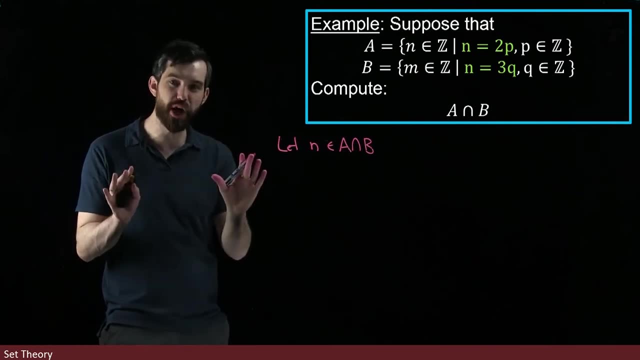 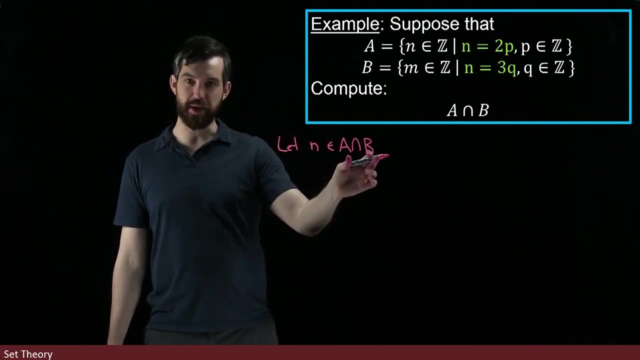 So I'm going to begin with, let my n be an element of A intersect B, So that's my starting assumption. and then, as we know, our next step is always applying definitions. So if n is in A intersect B, then it means it's. it's both in A and in B, but that means that it's a. 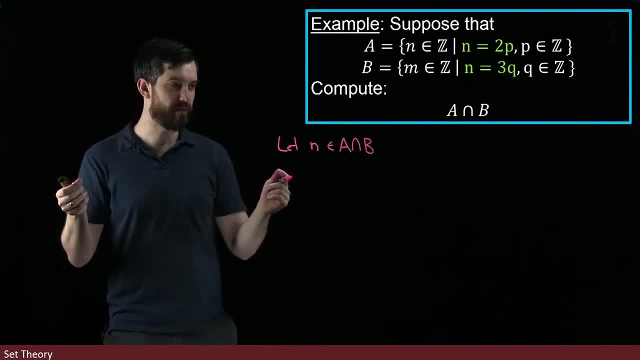 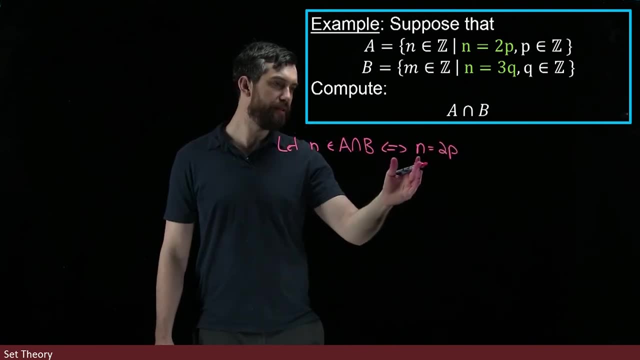 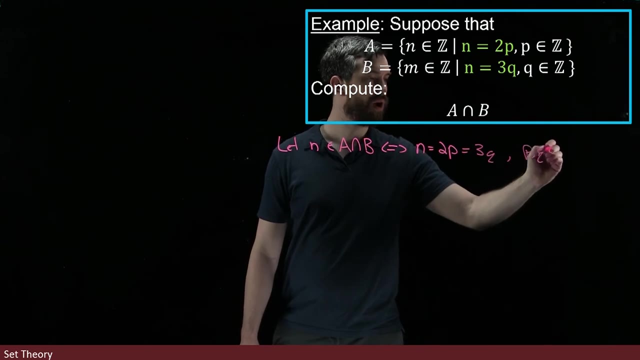 multiple of two and it's a multiple of three. So this is going to be the same thing as saying that n is equal to 2p, and then this is also equal to 3q, where the p and the q are inside of the integers. Now, if i focus on the, 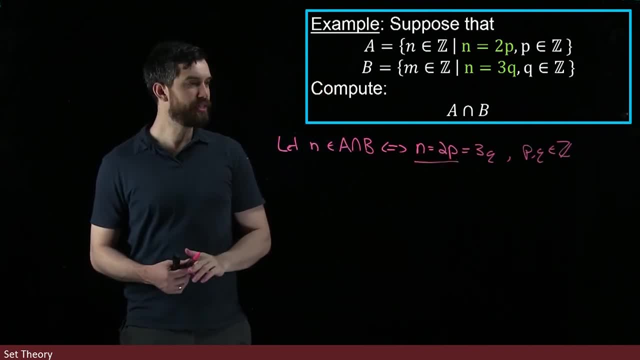 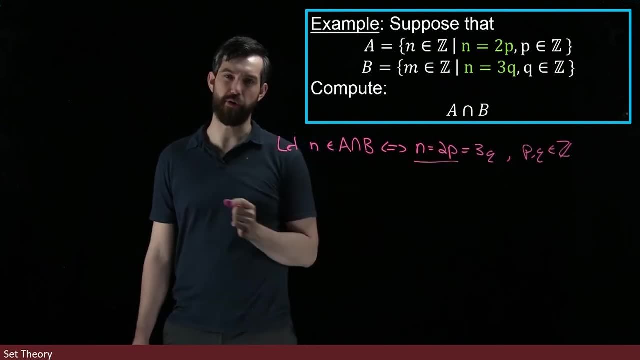 n equal to 2p. portion of this equation. notice that we're saying that if n is going to be a multiple of 3, then 2p is going to be a multiple of 3.. But clearly 2 isn't a multiple of 3.. That's. 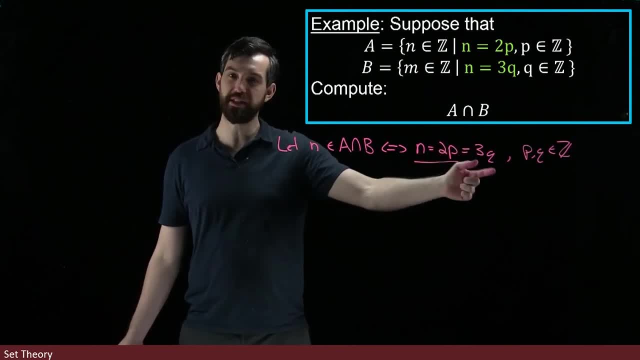 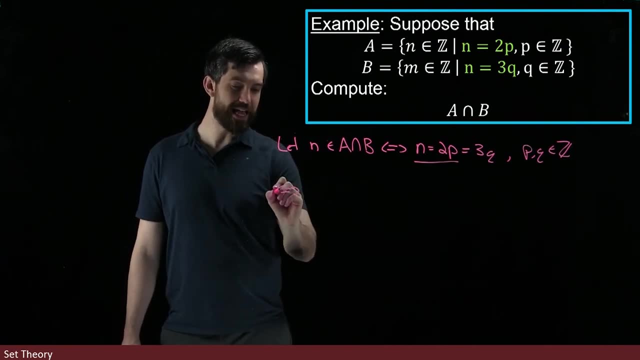 nonsense. So in this formula that 2p is a multiple of 3, it has to be that the p is a multiple of 3.. So in other words, this is the same thing as saying that this n here can be written in the: 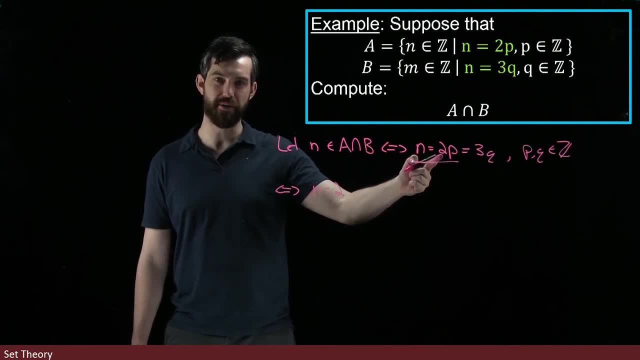 following way: It's the 2, and I'm taking this 2 here, But then the p itself is some multiple of 3. So this is going to be 2 times 3.. And then I've used up a p and a q, so I may as well put an. 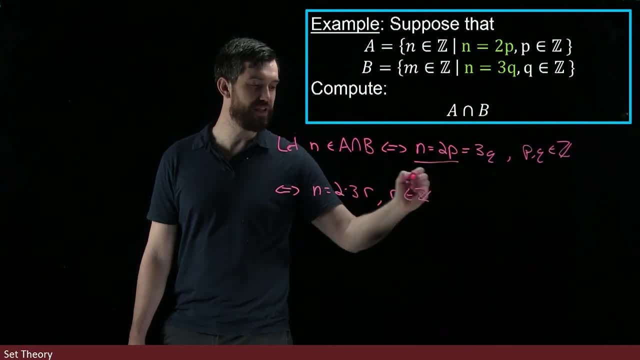 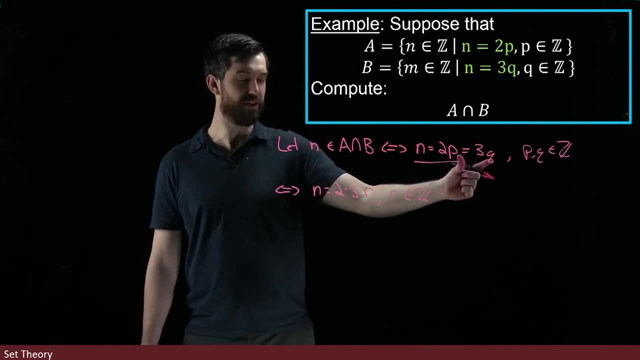 r here where r is going to be inside of the integers. So indeed, if n is equal to 2 times 3 times r, you can split it up into these two cases And if you have it split up you can put.